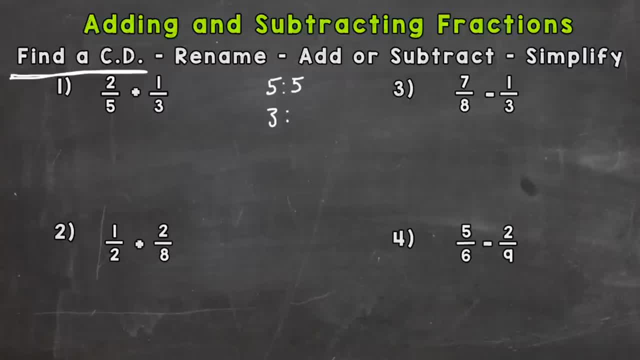 five will multiply into. So five times one is five, 10, 15, and 20. Now that list will go on forever. So my suggestion would be to write out three or four at a time. And if you don't get a match, then you can extend your lists. So three, we'll go three, six, nine, 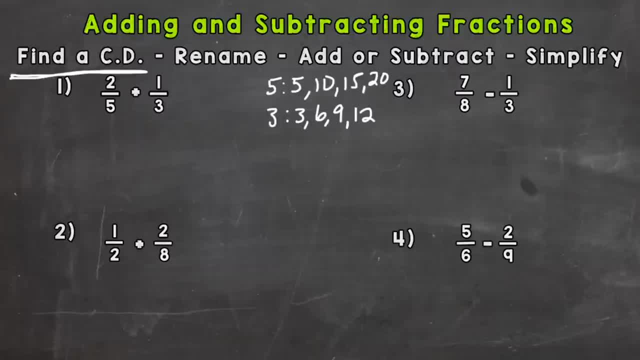 12. Now, we don't have a match for our multiples yet. So I'm going to extend the threes. And my next one, I'll get a 15. And we can see that 15 is our least common multiple here, the multiple that three and five share, that is the smallest in value. So we're going to use 15 for our denominator. So our next step 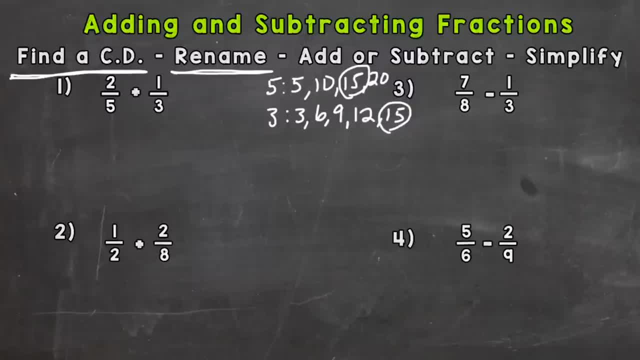 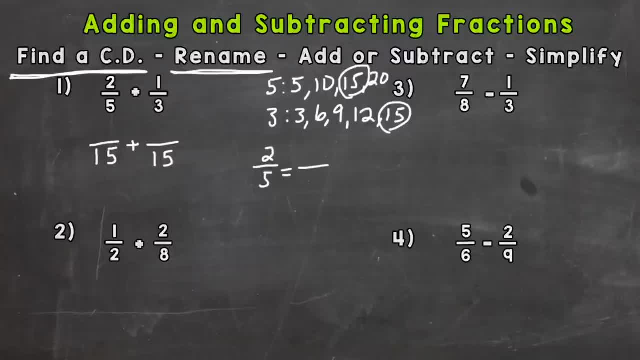 over here. And we need to find the equivalent fraction for two fifths. Now you set it up like this. And we have to see what we do to the bottom number that five to get it to equal 15. And we take that five times three, and it equals 15. So we need to do the same exact thing to the top, 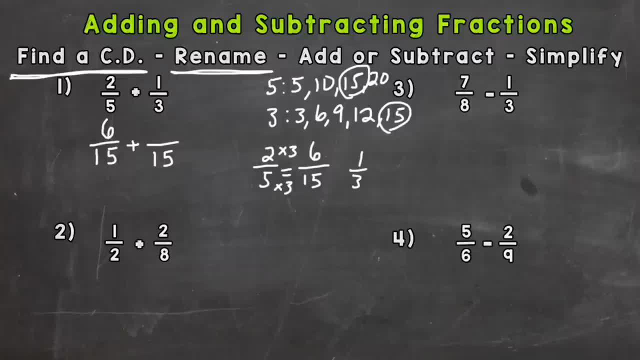 Now we need to do one third. So one third equals how many 15ths? Well, three times five is 15. So we need to do that same thing to the top. One times five is five. So this is going to be five 15ths. 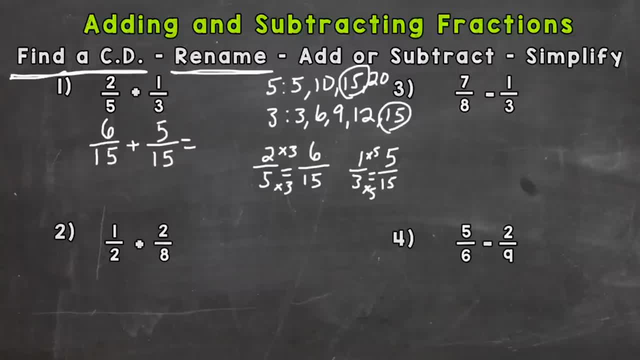 So now we found our common denominator here. We renamed with that common denominator. 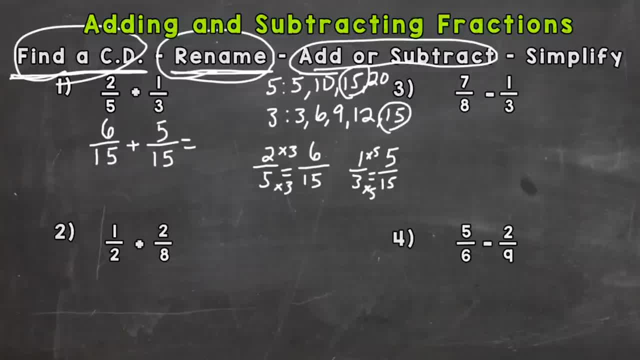 Now we're ready to add or subtract. And this problem's addition. So six plus five is 11. 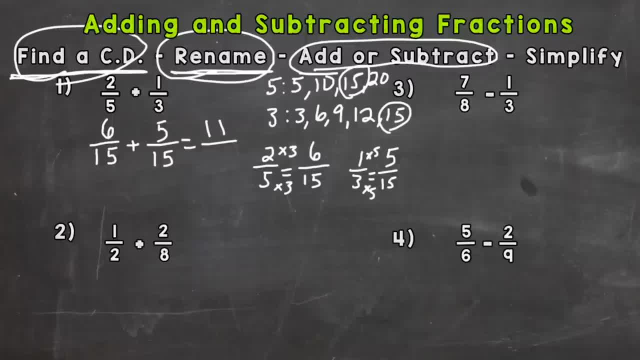 And then we keep our denominator the same. We do not do 15 plus 15. We keep it as is, 15. And lastly, we check to see if the denominator is the same as the denominator. So we check to see if the denominator is the same as the denominator. And lastly, we check to see if the denominator is the same as the denominator. And lastly, we check to see if the denominator is the same as the denominator. And lastly, we check to see if our fraction can be simplified or broken down. Now, are there any numbers that can divide out of both 11 and 15 to break this fraction down? 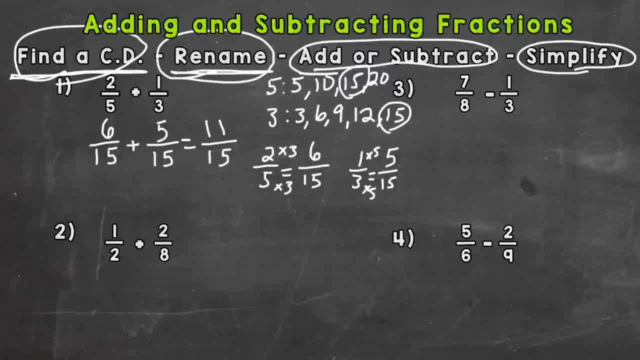 No, the only one is, uh, only common factor between 11 and 15 is one. So this fraction is simplified. We are done. 11 15ths would be your answer to number one. Now that seems like a lot of work and a lot of steps there. 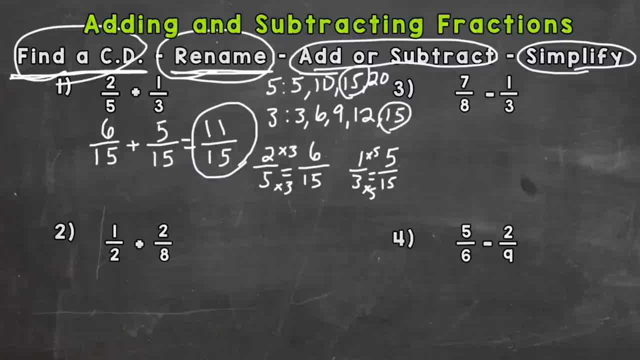 Now that seems like a lot of work and a lot of steps there. Now that seems like a lot of work and a lot of steps there. 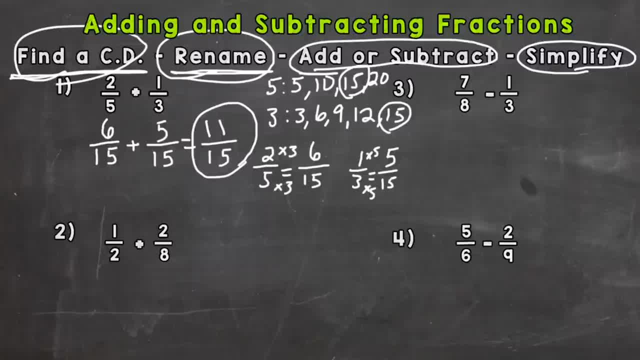 To, uh, get down, and just for a simple addition problem. But with practice and more experience, these go a lot quicker. 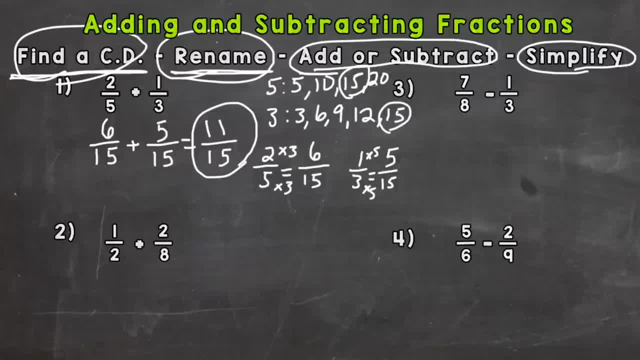 So let's go to number two. We have one half plus two eighths. So obviously our denominators are not the same. So we're going to need to find a common denominator. So we'll make our list for 2 and 8. Our multiples list. 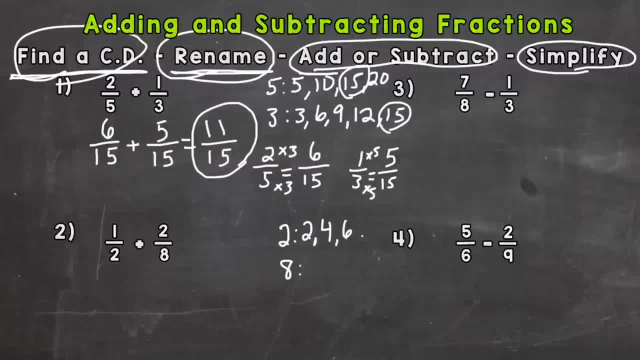 so two four six eight now let's make our list for eight well we start with eight and we should see a match so our least common multiple is eight so now we need to rename our fractions so I'm not going to go to the side for this one I'm just going to do it right below our original problem so I know this two I need to multiply by four to get a denominator of eight right two times 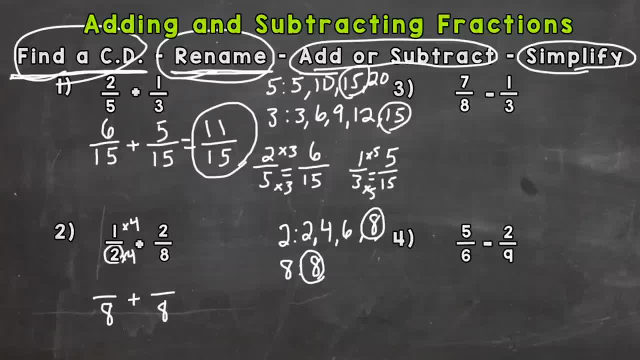 four so I need to do the same thing to the top one times four is four and as you can see here we have an equivalent fraction four eighths is the same thing as one half we're not changing the value when we rename we're just giving it a different name and a different denominator you 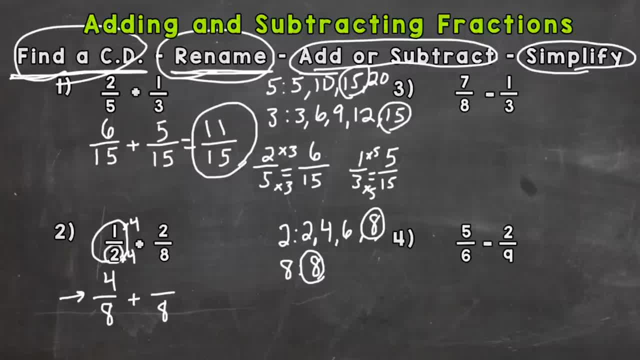 so we have a common denominator and we're able to add or subtract now two eighths already has a denominator of eight so we don't need to change that at all we are just going to bring the two down it already has a denominator of eight so we found a common denominator we renamed 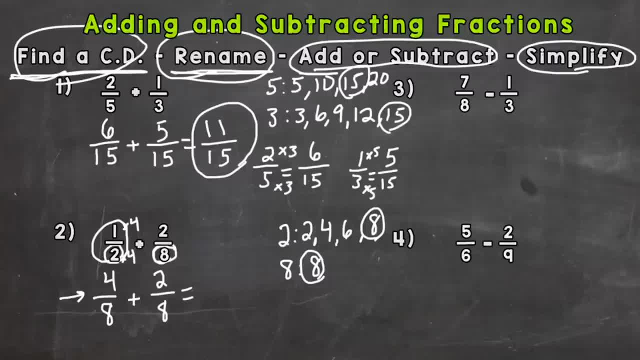 now we need to add or subtract so four plus two is six and we keep our denominator as eight now we need to simplify are there any numbers that can divide out of six 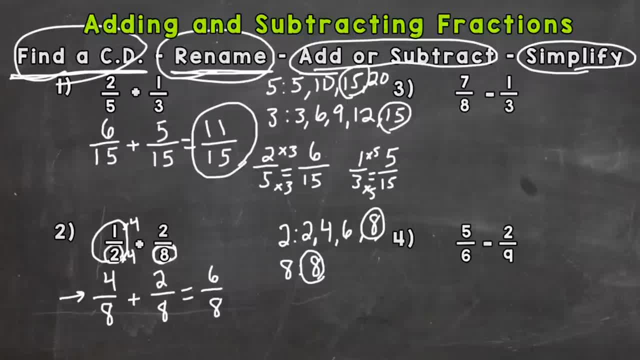 and eight any common factors to break this problem down yes they're both even and can be divided by two so we get six divided by two is three eight divided by two is four now the only common factor 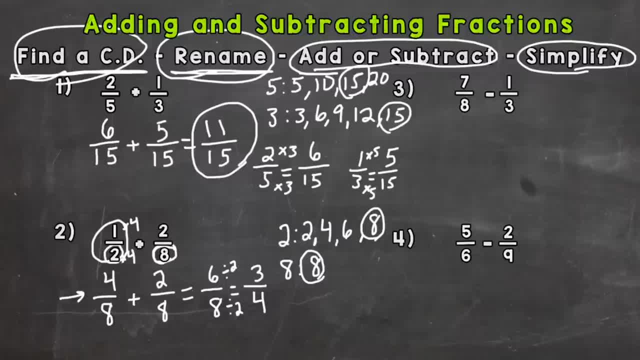 between that three and four is one that's the only thing that we can do to break this problem down so we are done the answer to number two is three fourths so let's go to number three we have a 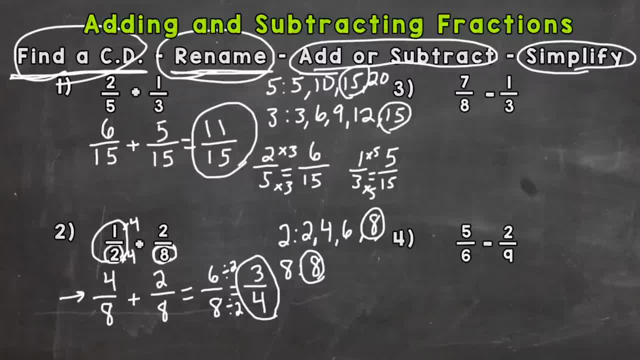 subtraction problem seven eighths minus one third here for number three so we obviously don't have a common denominator so our first step is going to be to find one so let's let's list our multiples for eight and three so eight sixteen twenty four thirty two now let's let's list our multiples of three three six nine twelve now we don't have a match yet so we need price to extend fifteen eighteen and I'm choosing to extend the threes because at the eight we're already to thirty two and there goes one third in喏w신了八,六夒、六四三十八,三十二,五七十八起,两十八 half a Milky Way revived on the obtaining or sturdy. Let's name three three three and let's list our numbers three three three three nine twelve now we don't have a match yet so we need to continue to extend fifteen eighteen and I'm choosingt the right the three is because that the eight we're already to thirtyso let's go to number fifty and let's go up and copy that and let's just go and provide the easy option here So we're going to extend our smaller list here. 21, 24. And we have a hit here with a common denominator of 24. So now we need to rename. 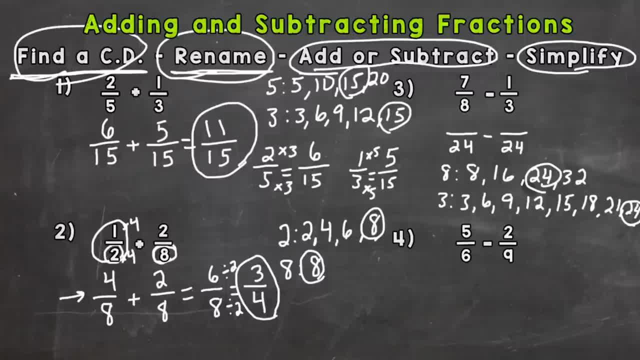 So 8 times 3 is 24. And 7 times 3 is 21. 3 times 8 gives us the denominator of 24. So 1 times 8 is 8. 21 minus 8 equals 13. And keep our denominator the same. The only common factor between 13 and 24 is 1. We cannot simplify or break that fraction down anymore. 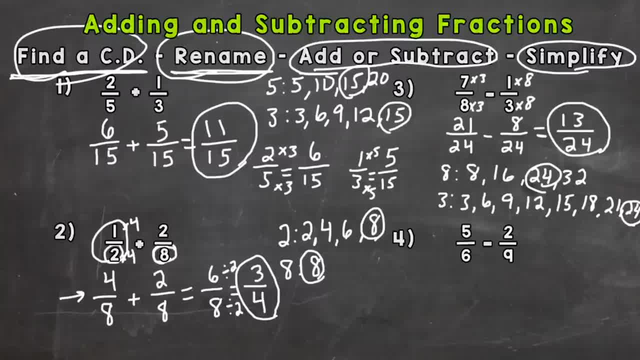 So our answer is 13 twenty-fourths. So subtraction is the same exact steps as addition. We just subtract instead of add. So number 4, we have a denominator of 6 and 9. 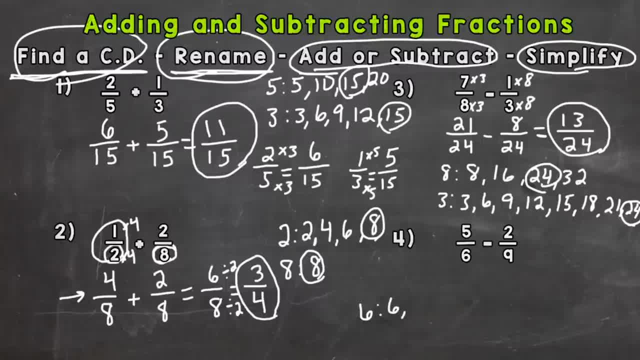 So we need to make our multiples list. 6, 12. 18, 24. 9. 9, 18. And we have a match. 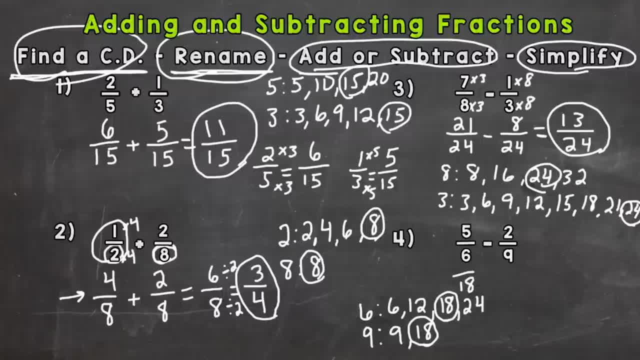 So our common denominator is going to be 18. 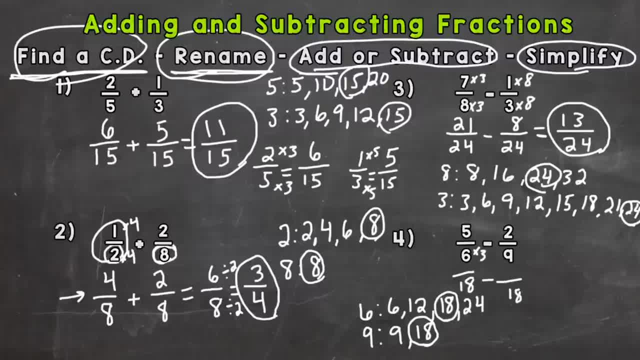 So 6 times 3 is 18. 5 times 3 is 15. 9 times 2 is 18. 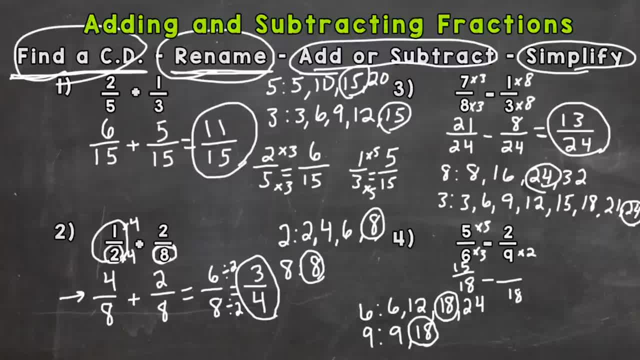 So we need to do the same exact thing to the top. So we have an equivalent fraction. 2 times 2 is 4. So we get to 15 eighteenths minus 4 eighteenths. And that gets us to 15 minus 4 is 11. Keep our common denominator of 18 the same. And we get to 11 eighteenths. Now 11 eighteenths does not have any common factors. 11 eighteenths does not have any common factors. Besides 1, we can't break that fraction down any further. So this is our final answer. 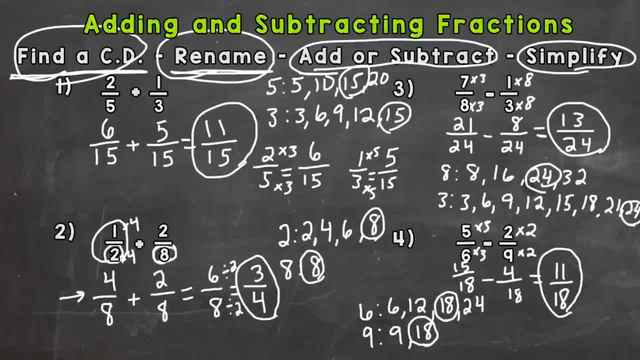 So there you have it. There's adding and subtracting fractions. Hopefully that helped out. 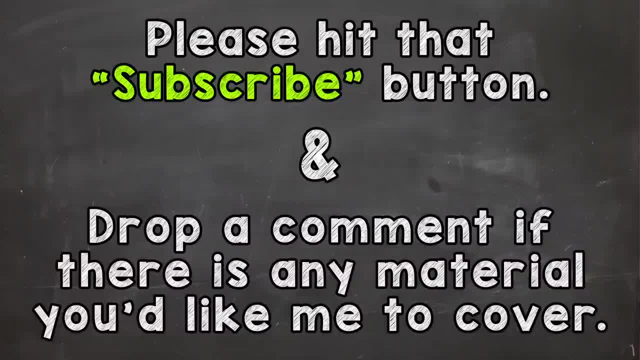 Thanks so much for watching. And until next time, peace.